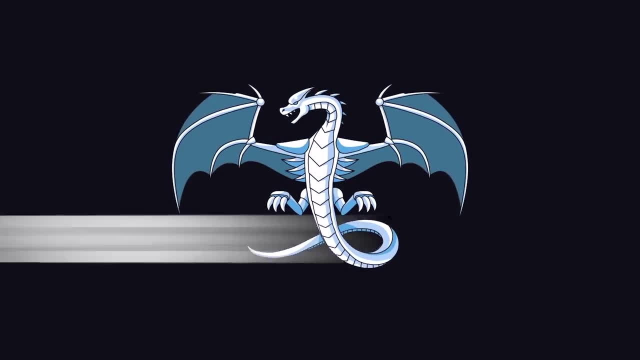 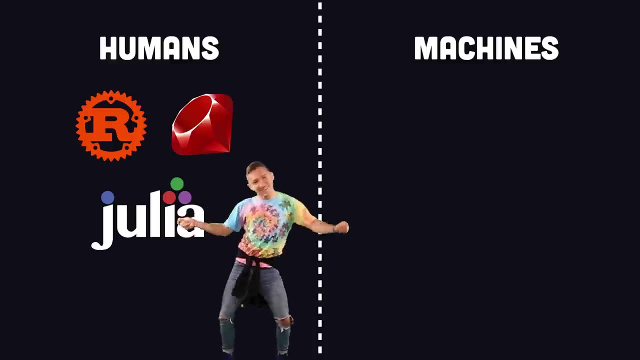 LLVM, a toolkit used to build and optimize compilers. Building a programming language from scratch is hard. You have humans who want to write code in a nice, simple syntax, then machines that need to run it on all sorts of architectures. LLVM standardizes the extremely. 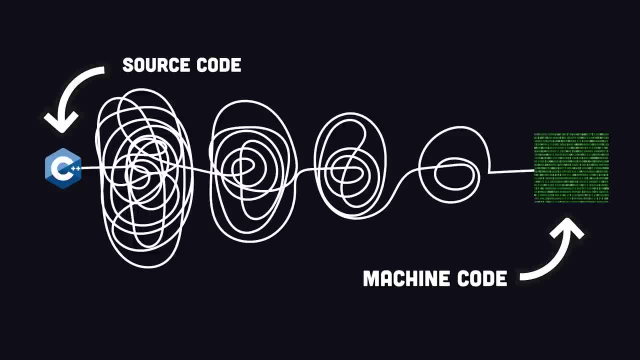 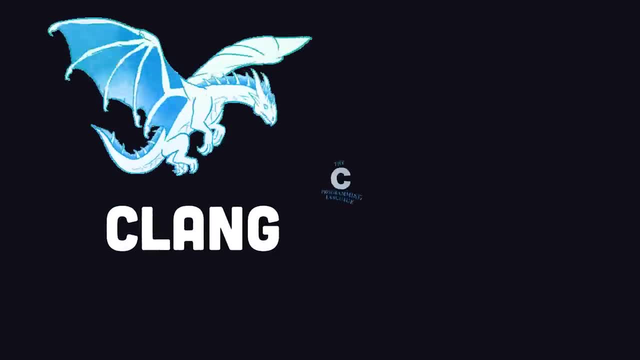 complex process of turning source code into machine code. It was created in 2003 by grad student Chris Lattner at the University of Illinois, and today it's the magic behind Clang for C and C++, as well as languages like Rust, Swift, Julia and many others. 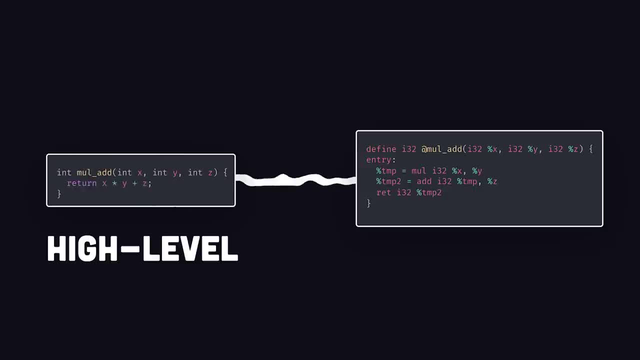 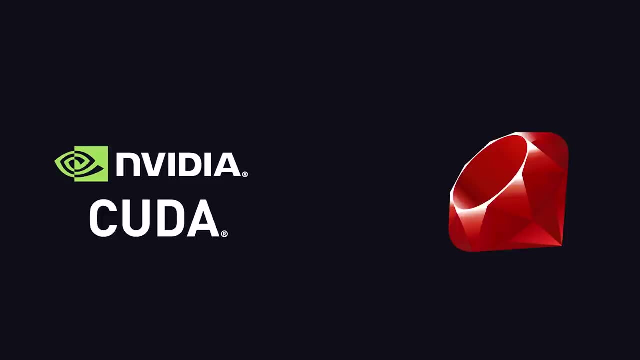 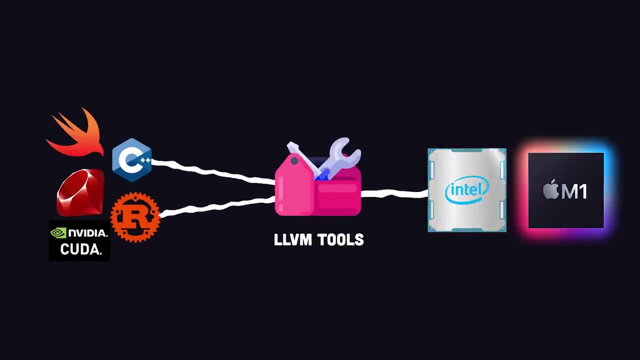 Most importantly, it represents high-level source code in a language agnostic code called Intermediate Representation or IR. This means vastly different languages like CUDA and Ruby produce the same IR, allowing them to share tools for analysis and optimization before they're converted to machine code. for a specific chip architecture, A compiler can be broken down into. 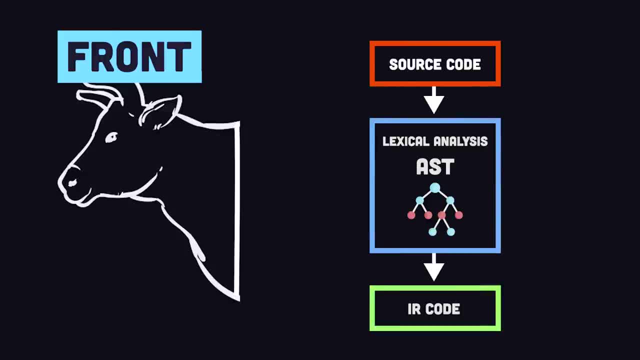 three parts. The front end parses the source code text and converts it into IR. The middle end parses the source code text and converts it into IR. The middle end parses the source code and analyzes and optimizes this generated code. And finally, the back end converts the IR into 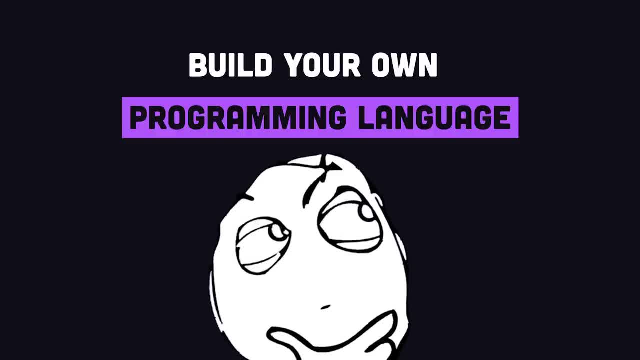 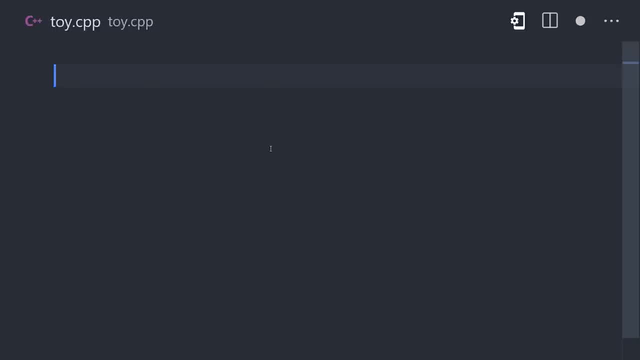 native machine code To build your own programming language from scratch right now. install LLVM, then create a C++ file. Now envision the programming language syntax of your dreams. To make that high-level code work, you'll first need to write a lexer to scan the raw source code. 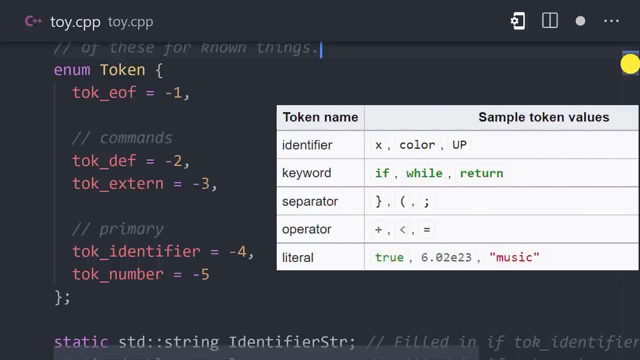 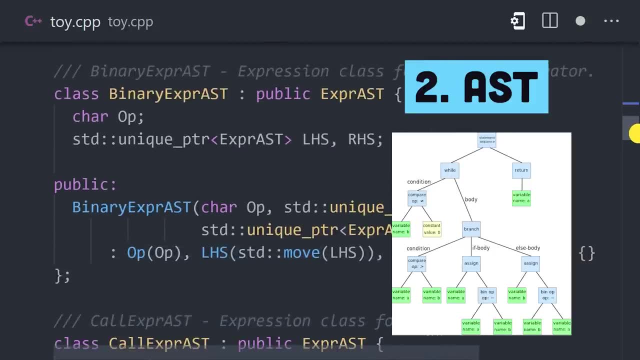 and break it into a collection of tokens like literals, identifiers, keywords, operators and so on. Next, we'll need to define an abstract syntax tree to represent the actual structure of the code and how different tokens can be used to create a new syntax tree. To do this, we'll need 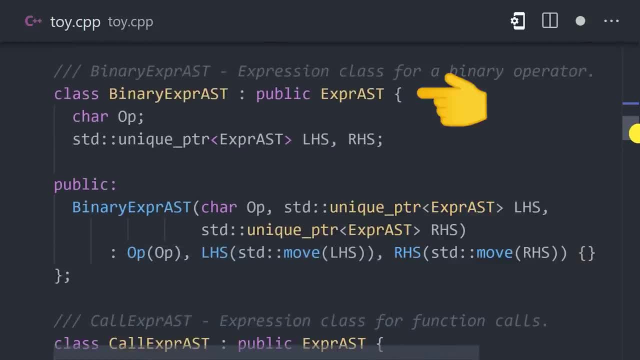 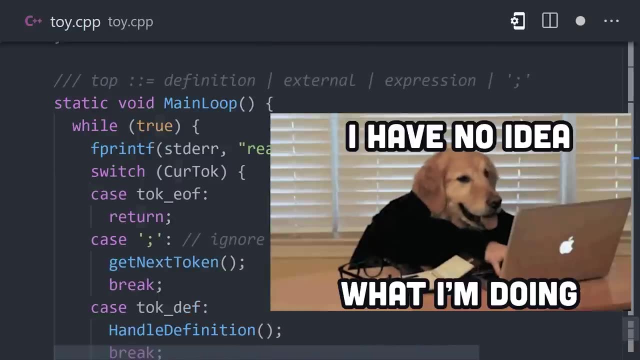 tokens relate to each other, which is accomplished by giving each node its own class. Third, we need a parser to loop over each token and build out the abstract syntax tree. If you made it this far, congratulations, because the hard part is over. Now we can import a bunch of LLVM primitives to 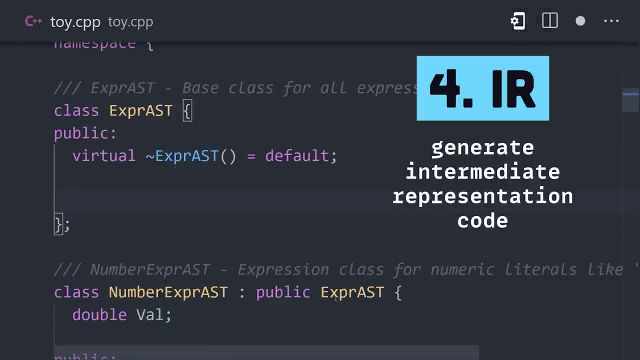 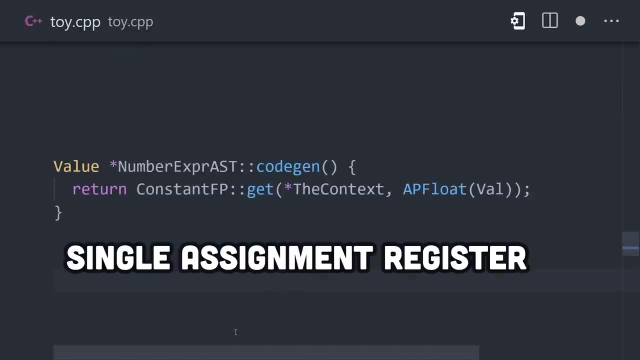 generate the intermediate representation. Each type in the abstract syntax tree is given a method called codegen, which always returns an LLVM value. object used to represent a single assignment register, which is a variable for the compiler that can only be assigned once. What's interesting? 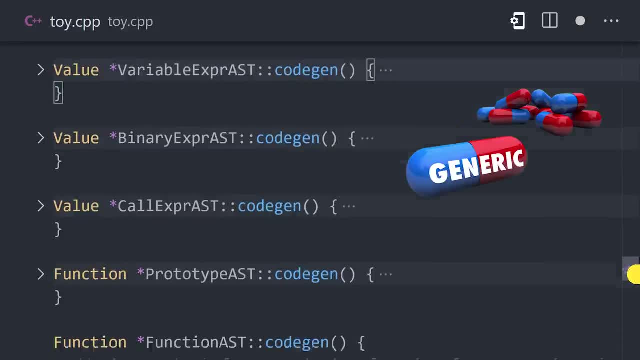 about these IR files is that they're not always the same. They're always the same, but they're all the same. The problem with LLVM primitives is that, unlike assembly, they're independent of any particular machine architecture, and that dramatically simplifies things for language.